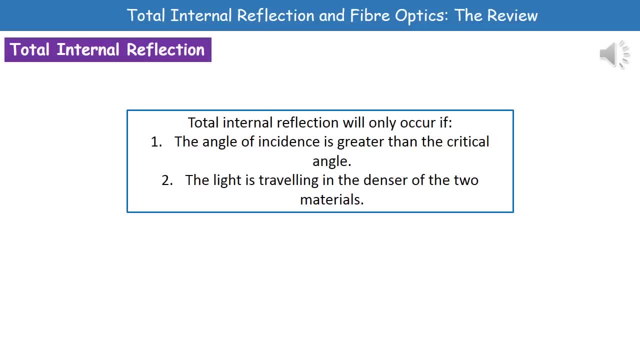 conditions that must happen for total internal reflection to occur. So first of all we've got to have an angle of instance greater than the critical angle, and the second thing is that the light is traveling in the denser of the two materials. So total internal reflection. 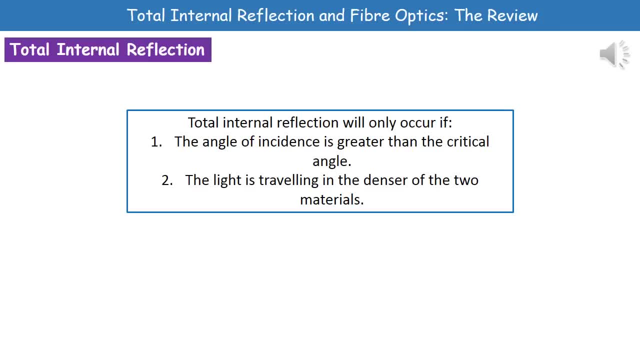 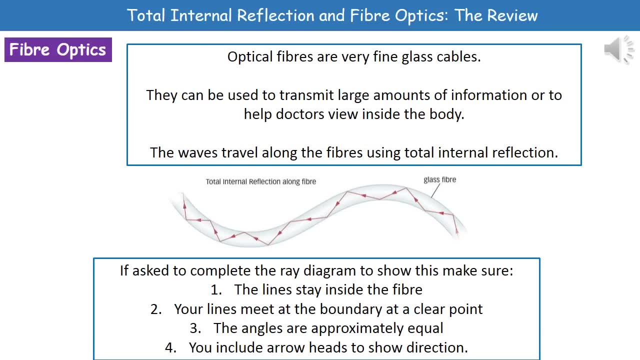 wouldn't happen if the light was traveling through the air and coming towards glass. It will only happen if it's traveling in the glass towards the air. Now we can actually use this idea of total internal reflection in fiber optics. So when we're talking about optical fibers, we're referring to 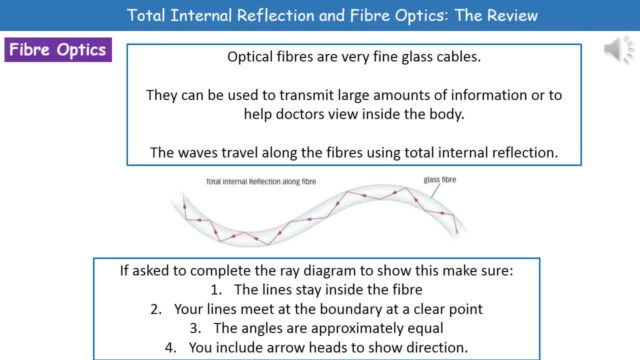 very, very fine glass cables and we can use these to transmit very large amounts of information, and we can also use them to view inside the body without having to have extensive surgery, And the way that it works is that those waves that we're actually transmitting are moving along the fibers. 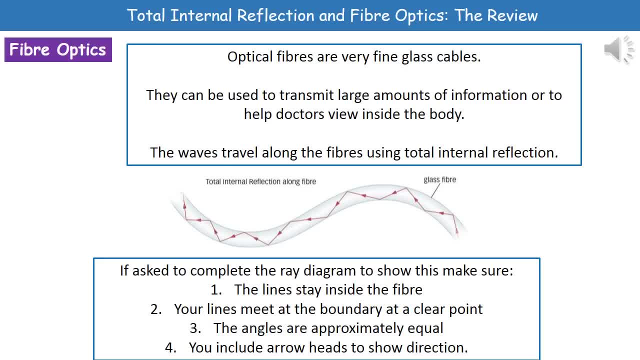 using total internal reflection. So I've given you a diagram there to show you how this actually works. Now I have seen them ask you to actually complete one of those ray diagrams before on the exam paper. So they will give you literally the starting point. They will give you the actual. 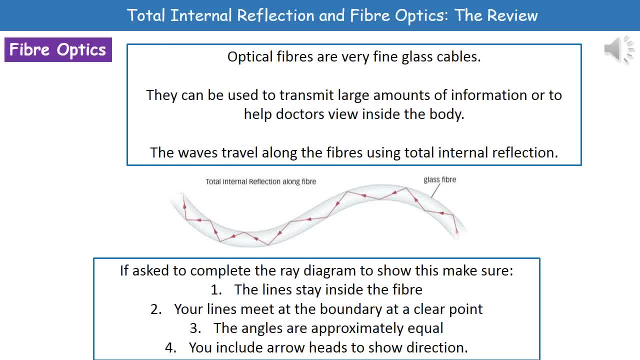 fiberglass and then you'll have to carry on that pattern. So if they ask you to complete this, make sure, number one, that your lines stay inside the fiber. Don't rush and have them then coming outside of the actual fiber itself. Also, make sure that your lines are meeting at that boundary at a very 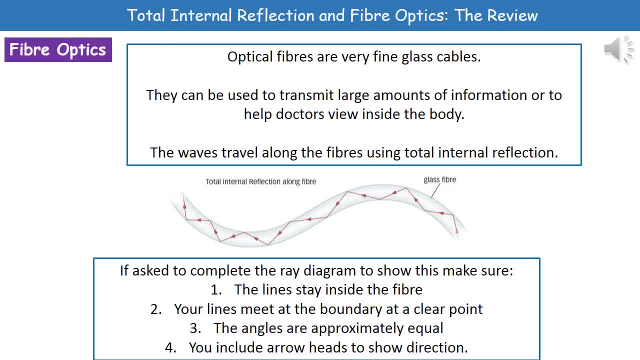 clear point. So don't have them crossing halfway, not actually managing to meet each other, etc. because you're going to lose a mark for that. You've got to make sure that your angles are approximately equal. Now you don't have to use a protractor, but just make sure that they do look. 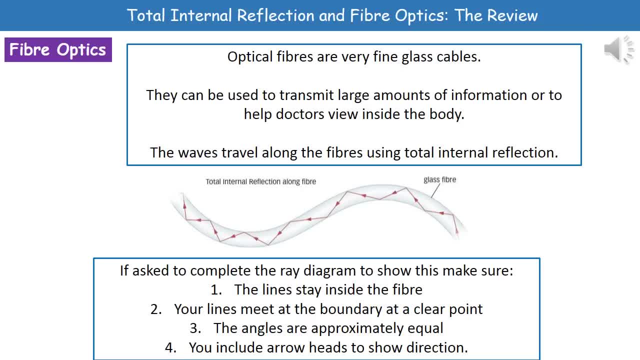 roughly equal. So don't have one that's a very, very small angle, another one that's a very large angle. Try to get them all looking roughly the same And then finally, make sure that you include the arrowhead to show the direction, as you should do with any ray diagram. So, in terms of the uses,